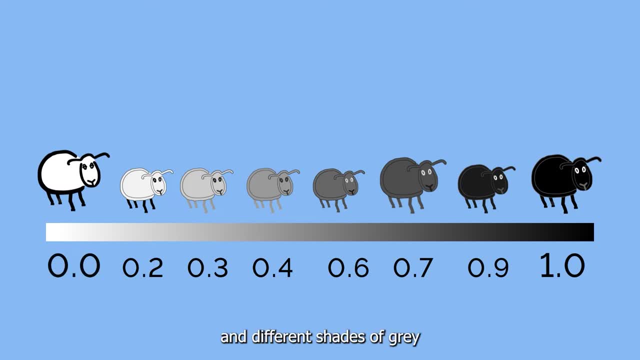 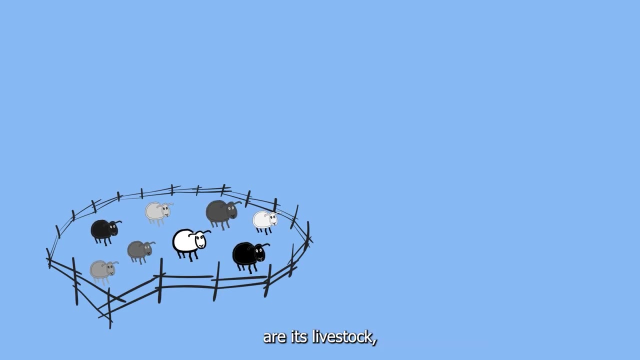 0, and a different shade of gray will get values that fall in between. A more elaborate example we can use is a sheep farm. Some of the key components of a sheep farm are its livestock, its meadows and pastures, but also the final products of animal farming. 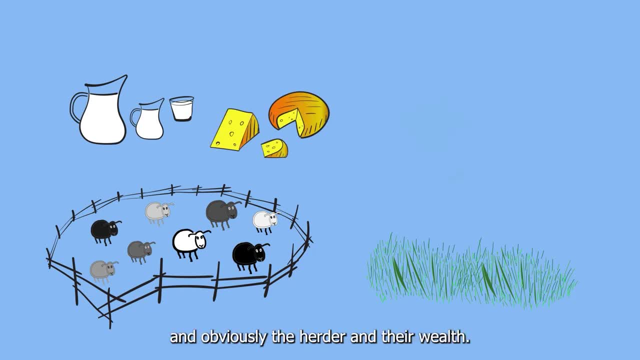 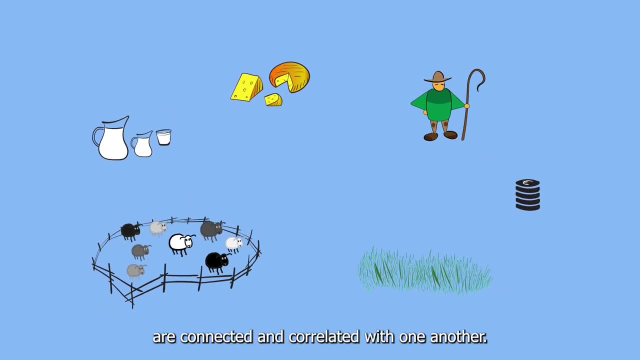 like milk or cheese, and obviously the herder and their wealth. All these components are connected and correlated with one another. For example, livestock and cheese are connected because cheese is produced with sheep milk. Using the fuzzy approach, we can define this connection to be very strong. 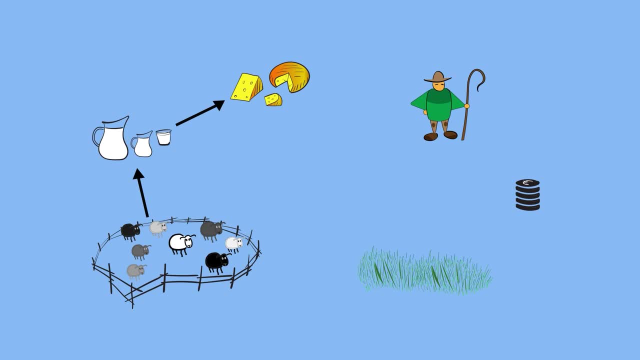 because without sheep there is no milk and without milk there is no cheese. Using a scale between 0 and 1, we can estimate a value of 0.8 for the relationship between the number of sheep and the amount of milk and cheese available. 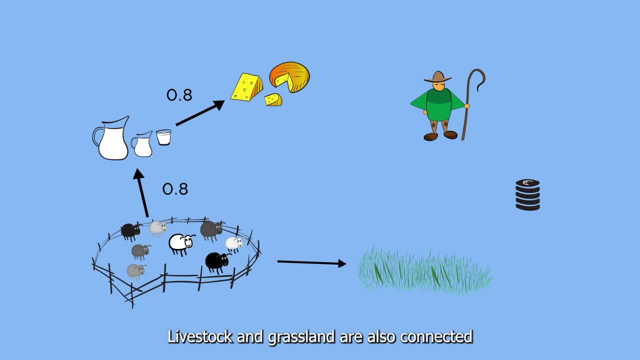 Livestock and grassland are also connected because animals eat grass. The connection is again quite strong because without grass there are no sheep. But, unlike in the previous example, the amount of grass decreases when the sheep graze. Therefore we should give the connection a high number but a negative value like minus 0.7.. 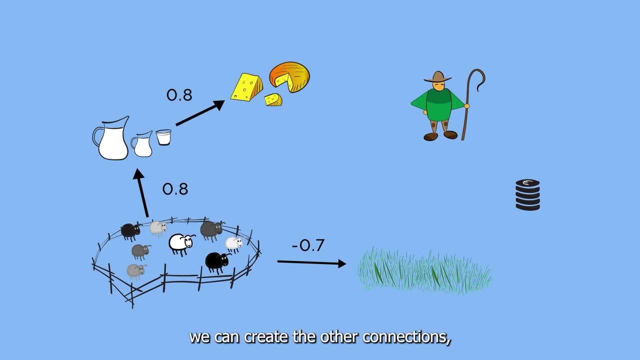 Following the same rationale, we can create the other connections, estimate their strength and decide if they are positive or negative. The connections are not only positive or negative, but are weighted based on their importance. This allows us to map the degree of correlation between different components in any complex system.